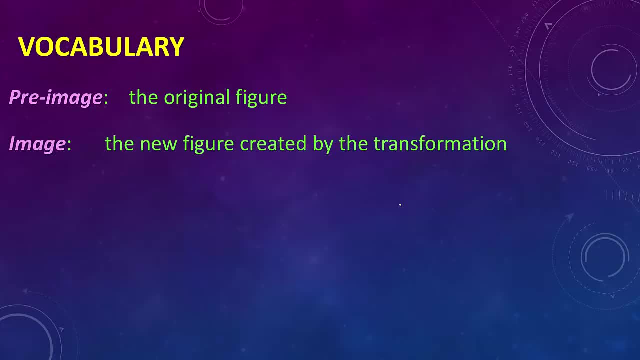 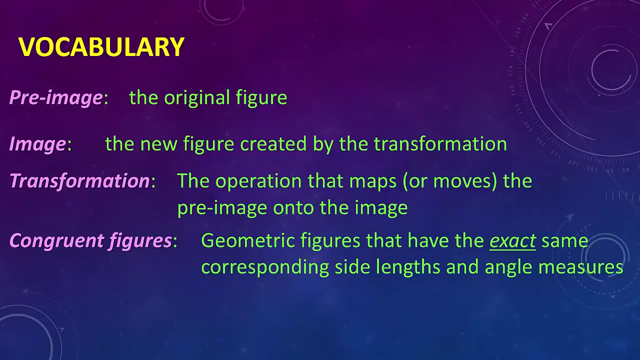 original figure. The image is the new figure created by the transformation. The transformation itself is the operation that maps or moves the pre-image onto the image. Congruent figures: these are geometric figures that have the exact same corresponding side lengths and angle measures. So what I mean by corresponding is, if I have a triangle, that 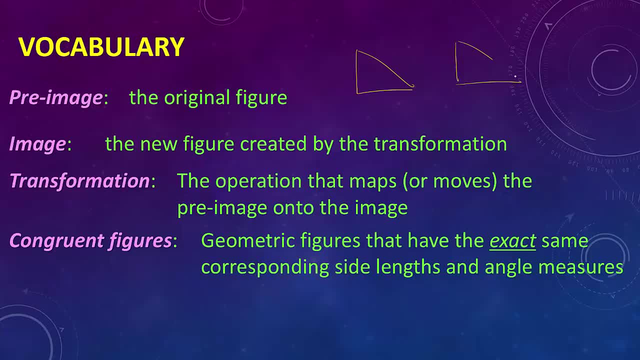 looks like this and I have another triangle. okay, and we're going to say, call this one ABC and we'll call this one DEF, And we're told that these two triangles are congruent. That means that if we're told the triangle ABC is congruent to triangle DEF, 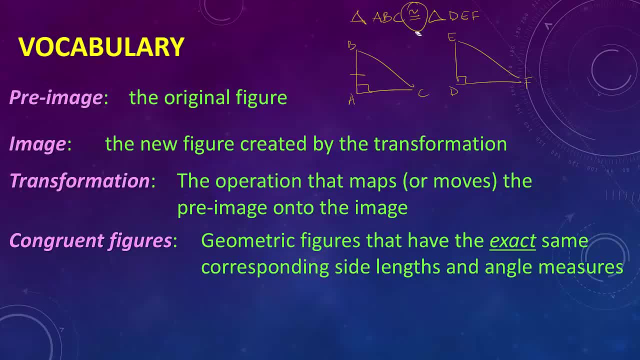 that's the symbol for congruent, So it looks like an equal sign, but it's got a little wavy symbol above it. Okay, so if A, if the order is ABC, so this, this and this, and then we're given DEF. 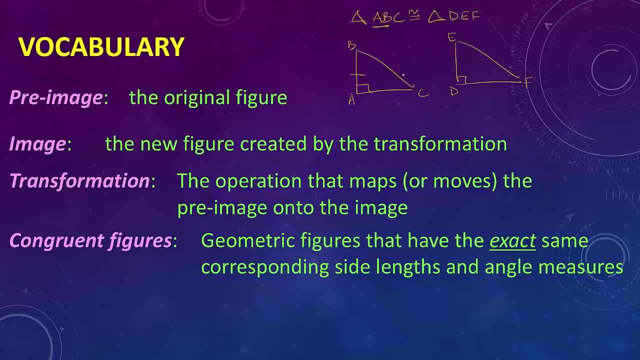 that means that, like, if you look at AB, that would be congruent to DE, so those parts would be congruent If you look at, say, BC, so this right here in the same spot in the naming. so the middle and third letter: the middle and third letter. 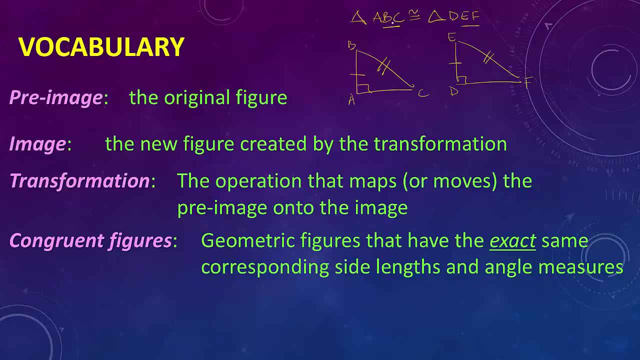 of the second one. so those parts are congruent. And then finally, if you took like the last two letters of each one, that would be the third congruent side. And then for angles, which we're really not going to get into a whole lot, this unit, but like angle B, would be congruent to 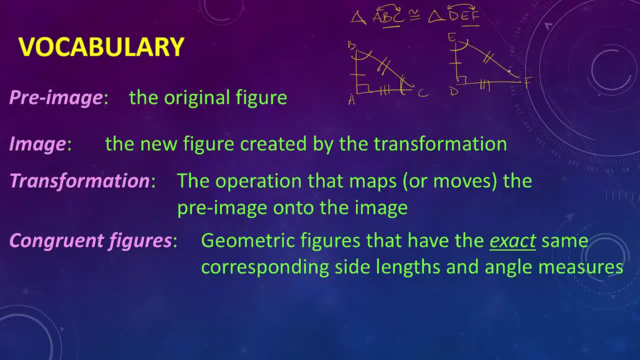 angle E, Angle C would be congruent to angle F. So you see, these marks are making those show congruence, All right, and congruent sides. those are corresponding sides of congruent figures that have the same measure or length. Okay, so that kind of gets into what I just showed. 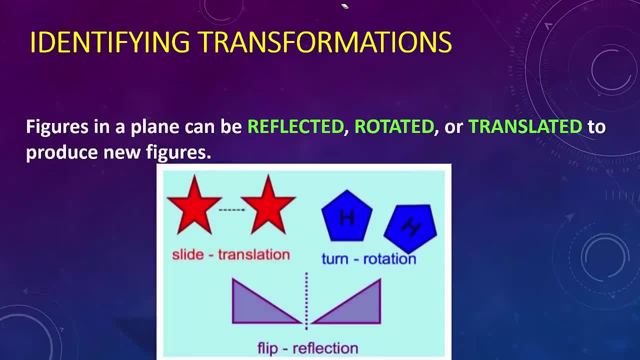 you, So first identifying transformations. Figures in a plane can be reflected, they can be rotated or they can be translated to produce new figures. So a translation would be basically taking the shape, keeping the exact orientation, meaning you don't turn it at all, you just slide. 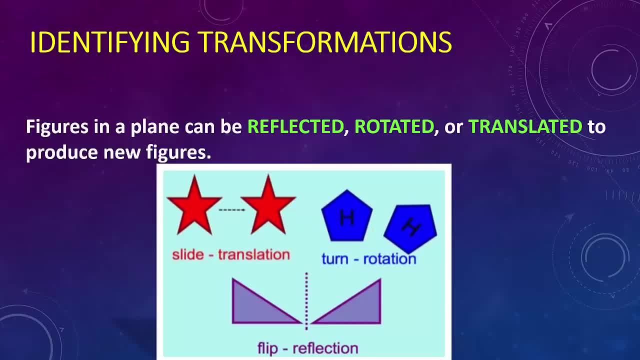 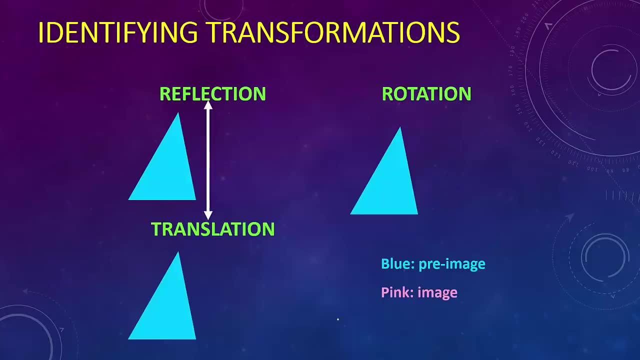 it left or right or up or down. Rotation can be described as a turn, so that see how we have the figure and it's turning, and then a flip would be the reflection. So if you have a line, you basically it'd be like looking in a mirror. you flip it over that, All right. so here's how they. 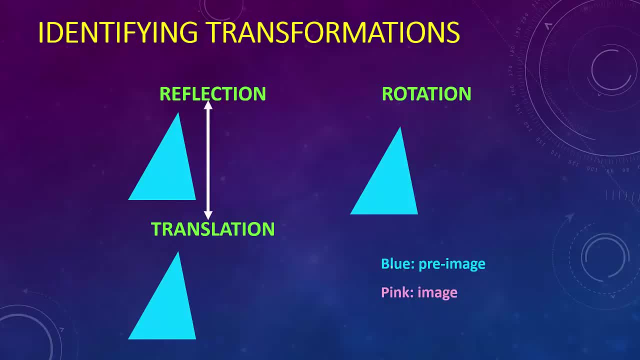 look. So a reflection. so the blue image would be the pre-image, the pink would be the image. so what results after the transformation? So reflection, see how it kind of flips over that line until it finally looks like that. and it should be noted that whatever it's being reflected over, like this distance here and this distance, 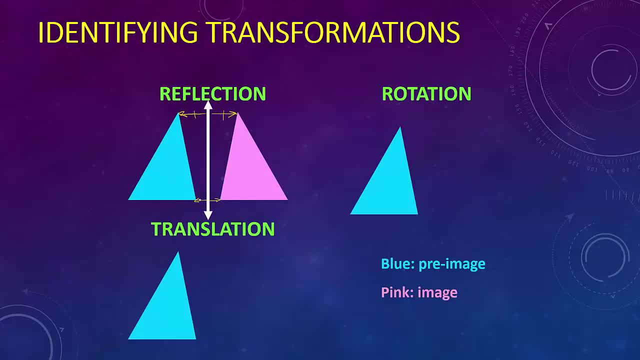 these would be the same distance, The distance between these two points- same distance, and then the distance from here to the ends. those are the same distance. Okay, translation would be: if you just took the figure and like that would be a slide right and then up and then rotation would. 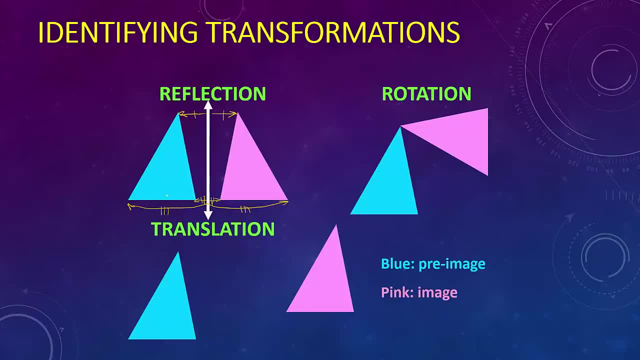 be like if I took it and rotated that 90 degrees Counterclockwise. so remember, clockwise like a hands of a clock, that's clockwise. counterclockwise would go like that. So that's important to know because if you're given a transformation or a 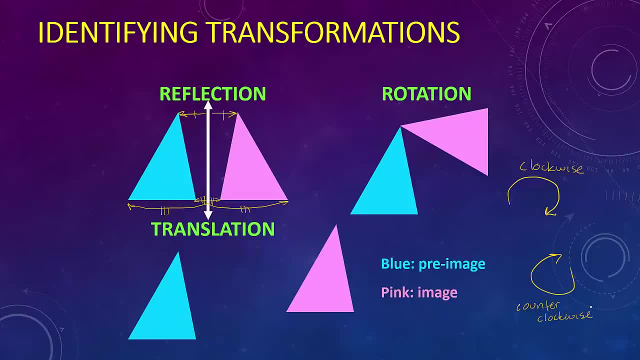 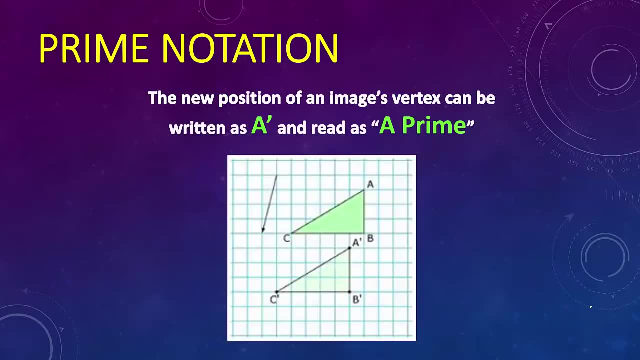 rotation, and you're told it rotates a certain amount of degrees, clockwise or counterclockwise. that could make a difference in how the final image looks. And then prime notation. so the new position of an image's vertex can be written as A prime and we call it, we basically read it as A prime. So if this is our pre-image here, 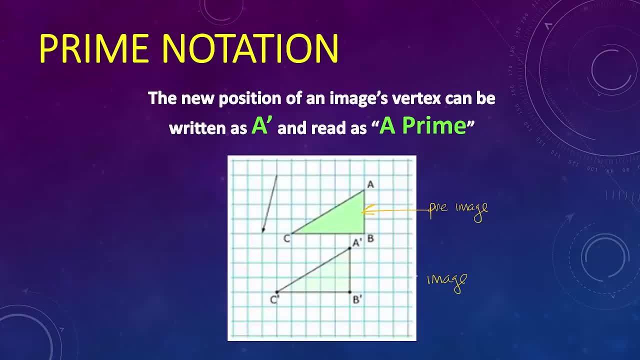 and we're using the same letters instead of different ones to differentiate between the pre-image and the image. we would just add a like an apostrophe, So it's. we call that prime notation. So this is the original image. the new image is a. you know this one here, an. 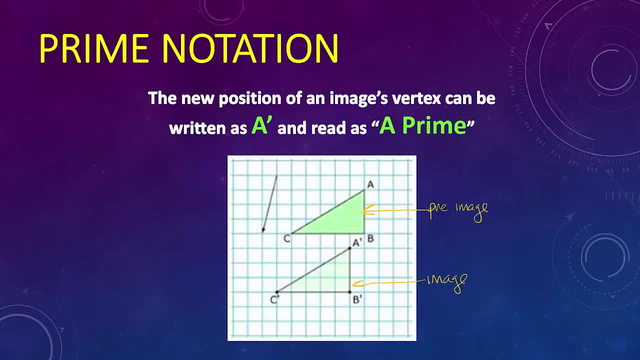 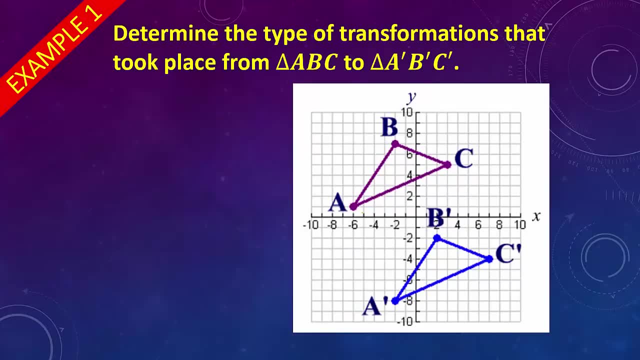 each vertex that corresponds now has this prime notation after it. So let's take a look at our first example. So we need to- all we need to do is determine the type of transformation or transformations that took place from triangle ABC to triangle A prime, B prime, C prime. 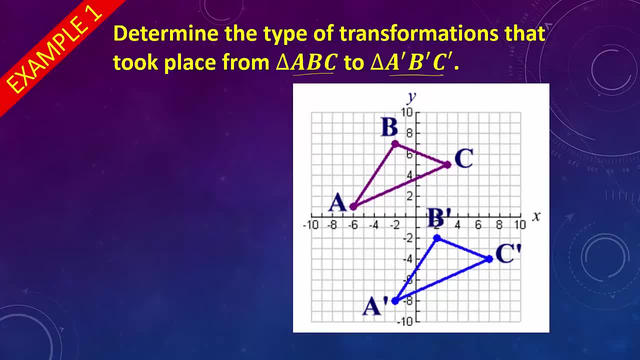 So it's important to note the notation that they use so you know which triangle you're starting at and going to Now. here, all we're doing is asking you to identify the type of transformation. So, in this case, notice how the B and the C have the same orientation. the figures look. 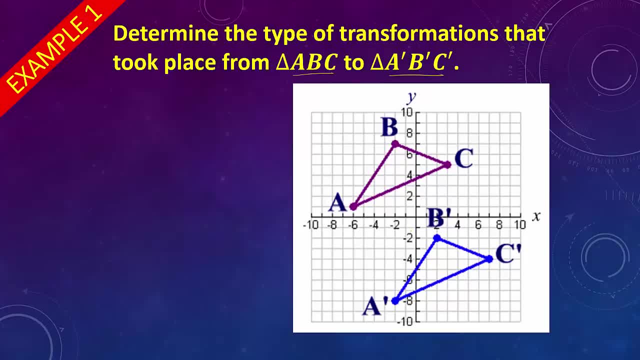 like if I took this one and moved it on top or vice versa, that they would be exact matches. So that would just be a slide, and if we were going to be specific, that would be a translation that would be slid down and then you would count like if it asked for an exact measure. 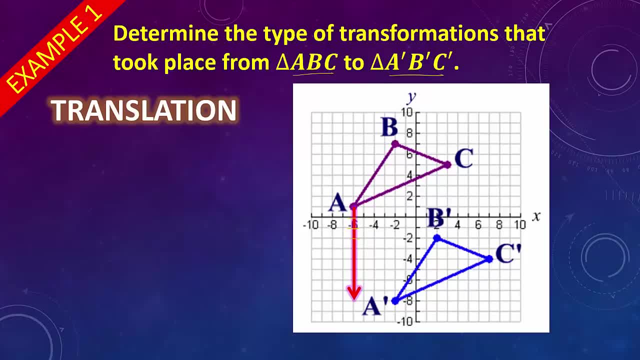 so it would be down 1,, 2,, 3,, 4,, 5,, 6,, 7,, 8,, 9.. So it would be down 9.. And then we'd count 1,, 2,, 3,, 4 to the right, and all you do is you find the corresponding. 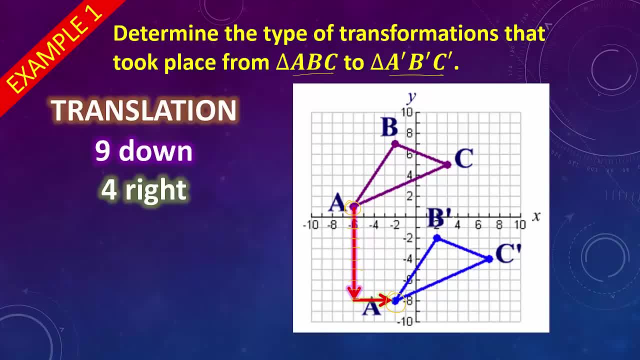 points and you only need to do it once. So we don't need to do it for B and C, because they would be exactly the same. So you just need to go from one point to the other matching point, So you wouldn't go from A to B prime, you'd go from A to A prime or from B to B prime. 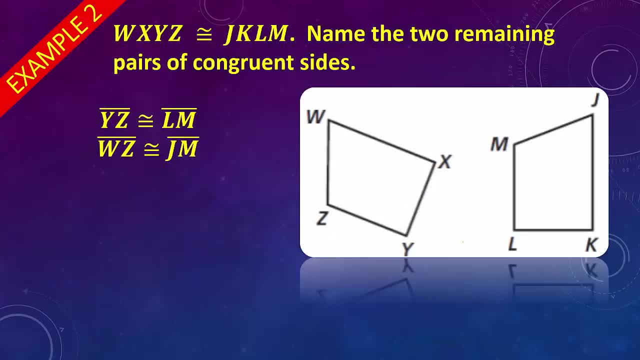 or from C to C prime. Alright, So now, As far as congruence goes, remember what I said is that congruence is when the corresponding parts have the same measure. So we're told that W, X, Y, Z is congruent to J, K, L, M. 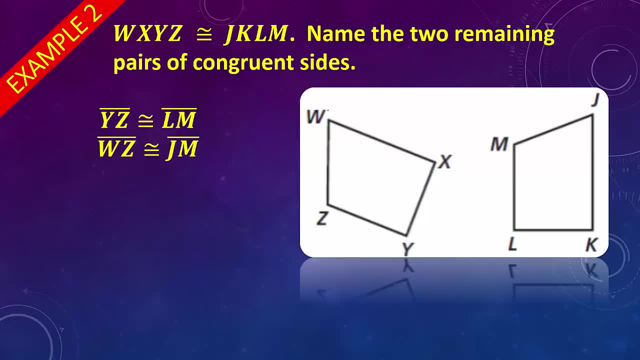 So let's just what I would suggest doing until you get the hang of this, is okay. so this is our first, second, third and fourth, and then go through. J is first, K is second, L is third and M is fourth. 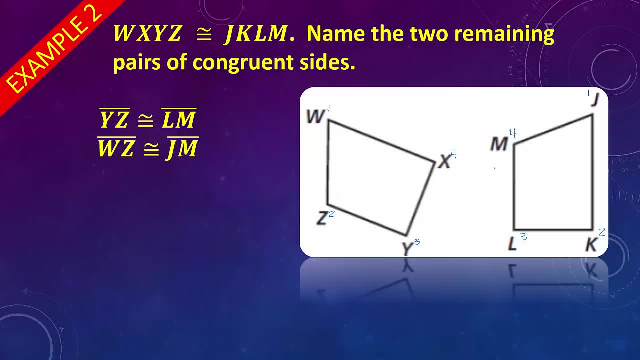 Okay, So now what you need to be careful of: we're told that Y Z is congruent to L M and we're told that W Z is congruent to J M. So you don't want to make any assumptions and say, well, you know, based on this, then 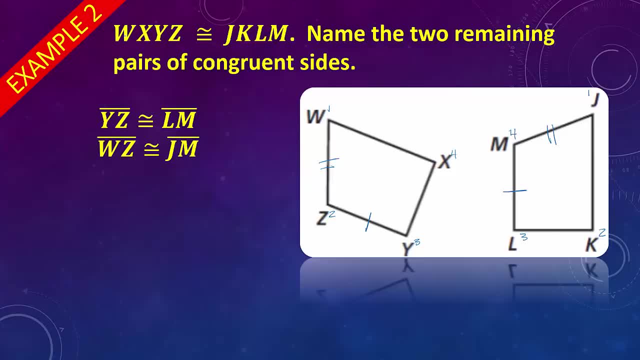 this has got to be the congruent part. Obviously, this figure has been rotated, so pay attention to how these are. So you can go back and, like you have that number, You can say: okay, so this is one, two, three, four, and over here we have one, two, three.